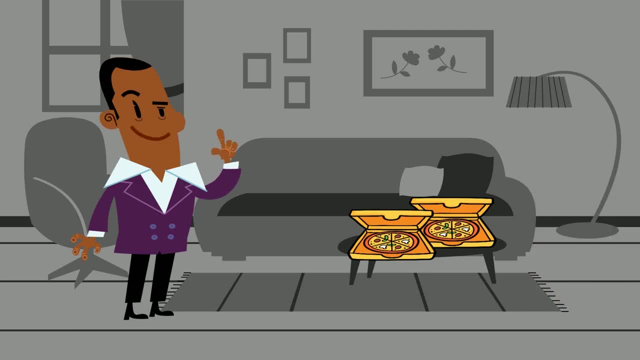 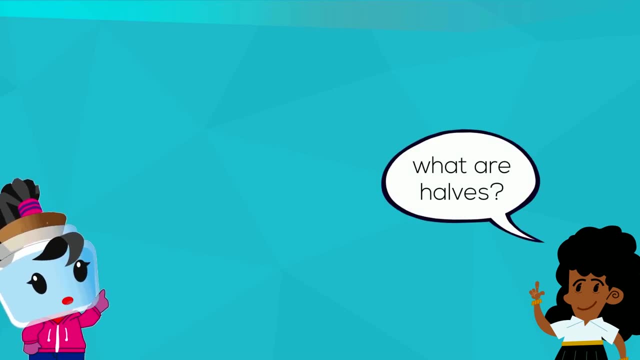 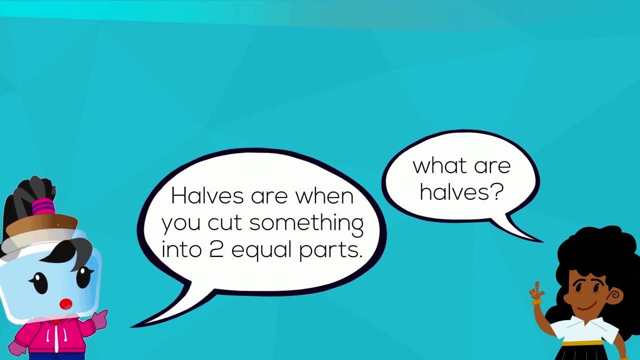 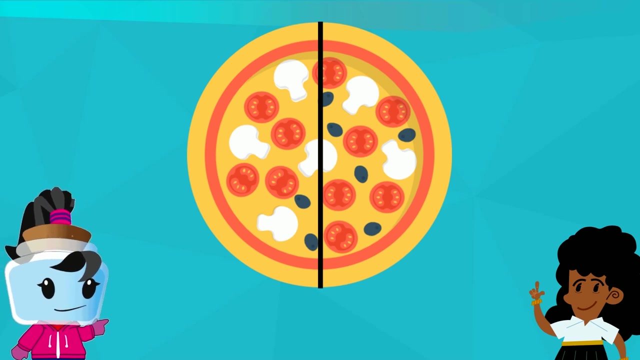 She's not quite sure how to do that, So that's why we're here to help. Sarah is wondering what halves are. Let's tell her: When you cut something into two equal parts, these two parts are called halves. Look, Sarah gets it now. She's slicing the first pizza into two equal parts. 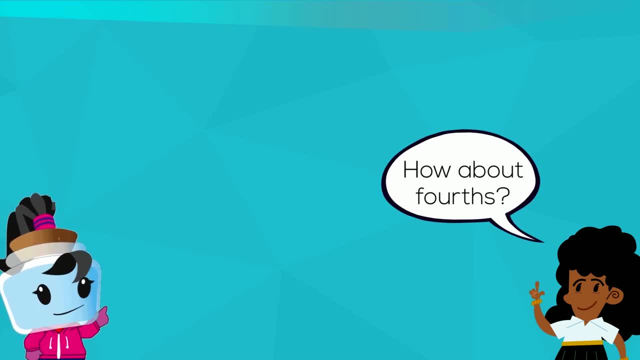 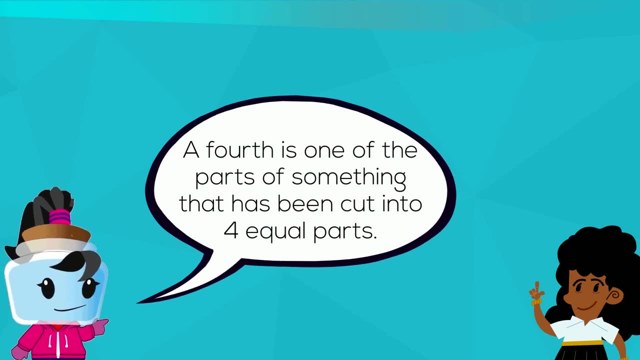 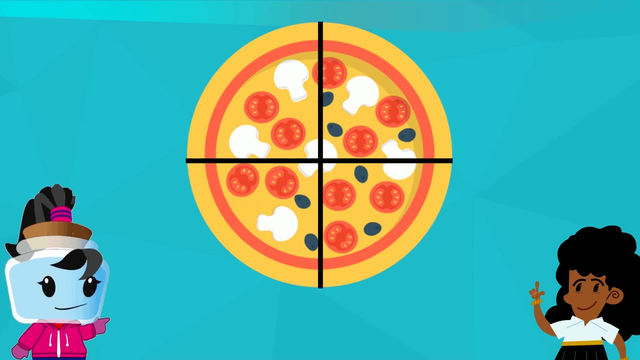 Now she wants to know what fourths are. Let's help her out again. A fourth is one of the parts of something that has been cut into four equal parts. Look at that. Sarah has cut the second pizza into four equal parts. Great job, Sarah. 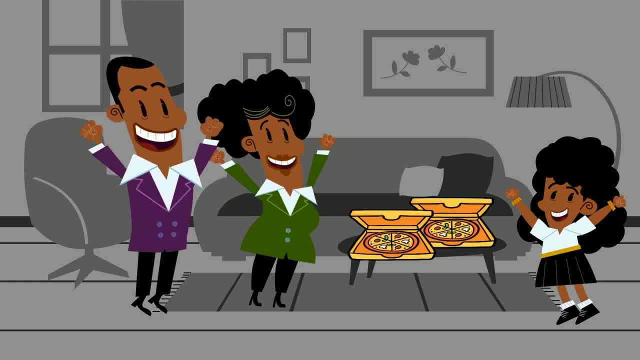 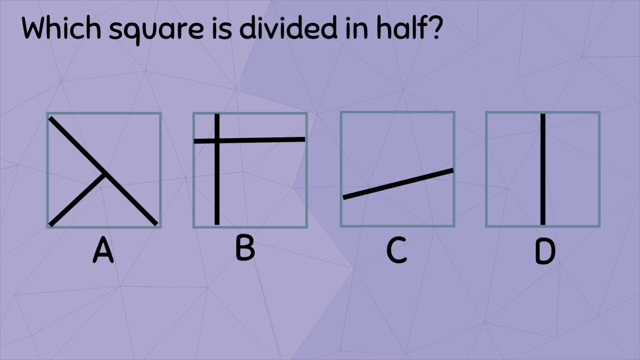 Now Sarah and her family can all eat the pizza. For more practice, let's look at these squares over here. Try to guess which one of them is divided in half. Remember that half means being divided into two equal parts. That's right. It's square D. 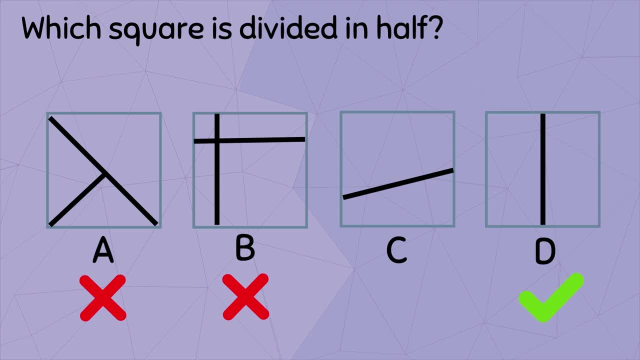 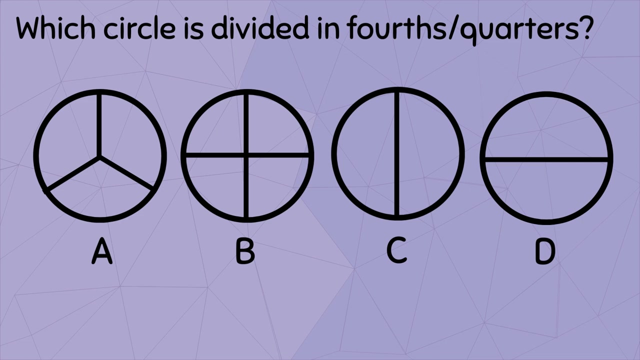 Both square A and B are not divided into two parts. Square C is divided into two parts, but the parts are not equal, While square D has two parts that have the same exact size. Let's move on to these circles. This time, let's find the circle that's divided into fourths, which can also be called quarters. 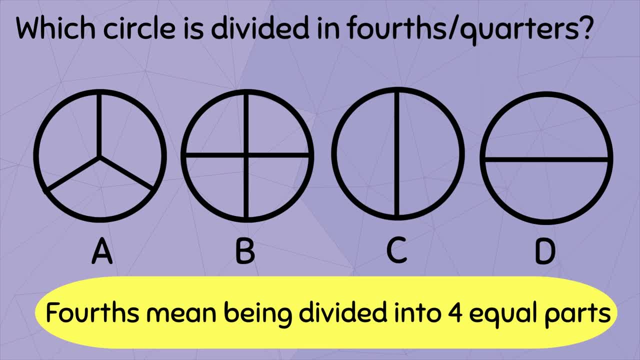 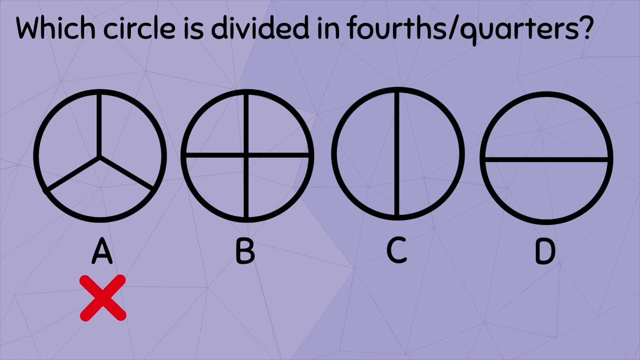 As long as it's divided into four equal parts. that's what we're looking for. Circle A is divided into three parts, So that's a. no, Circle B is divided into four parts that are all equal. So this is correct. The other two circles are divided in two equal parts.